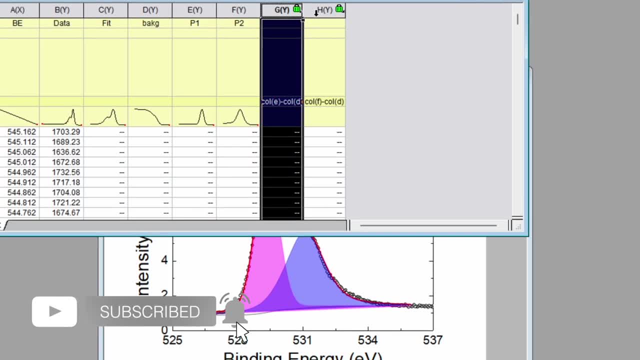 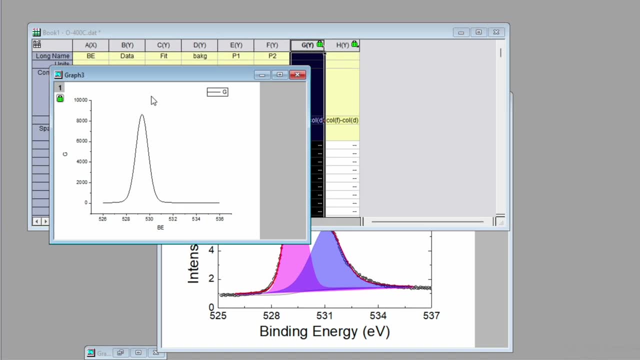 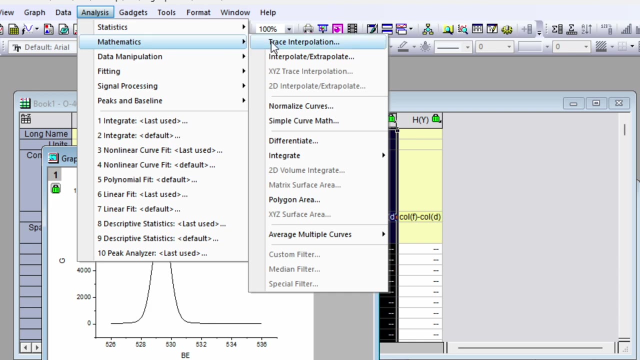 So apply and okay, Now we got these peaks. So click on the line and this is the peak P1.. Now, if you want to get the integrated area or area of this peak, what you need to go to the analysis, Then go to the mathematics. In this mathematics you can find all the 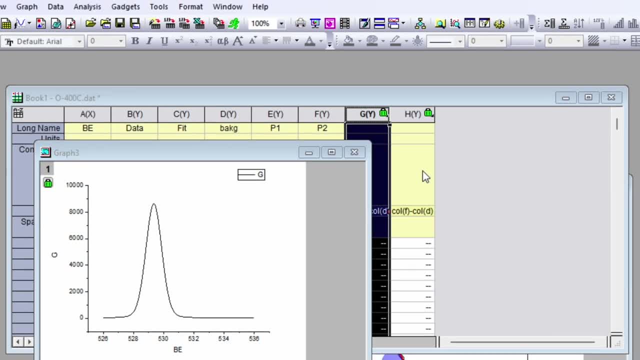 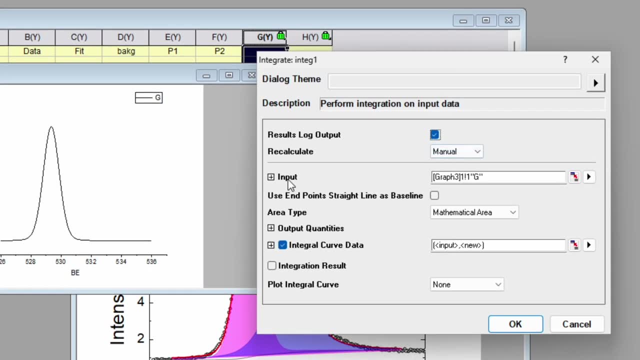 options for the integrated. Click on the open dialog. In the open dialog it will show result. log output: Yes. Recalculate manual input. So this is the data. Use endpoint straight line as a baseline. Click yes, Check this box and then area type Instead of mathematical. 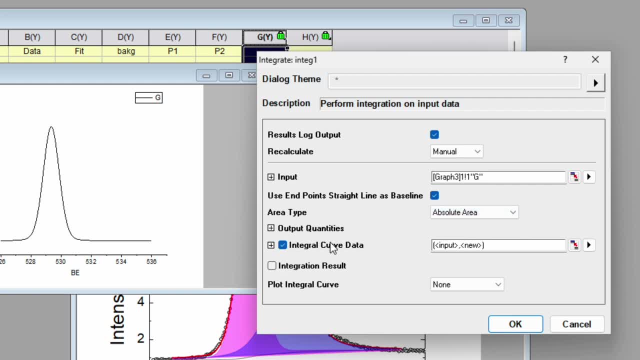 area. you can choose the absolute area, That output and keep all things as it is and just click okay, So it will automatically perform the integration. So this is the output. Now we need to calculate the output. So this is the output. So this is the output. So this is the output. So this 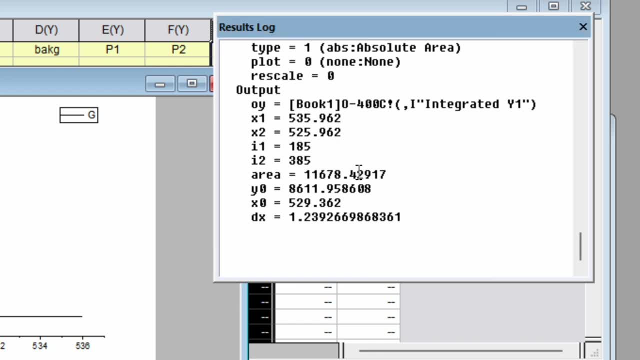 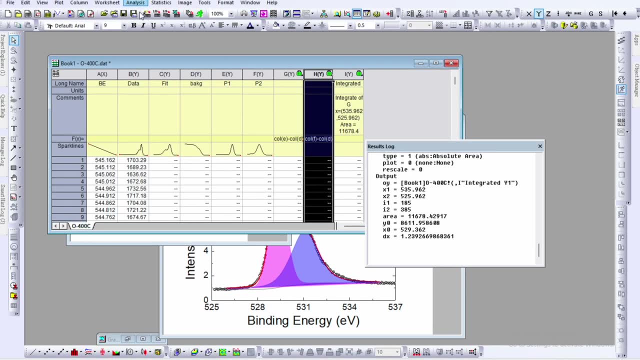 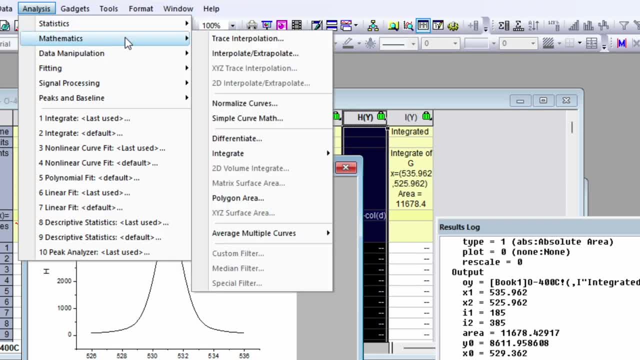 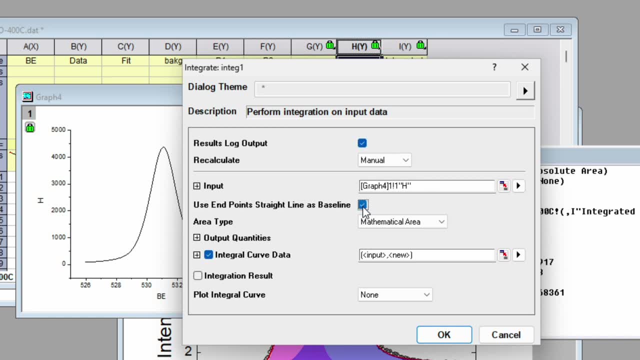 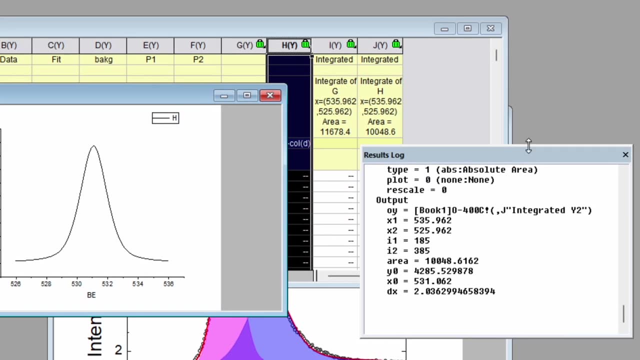 Line plot. Go to the analysis- Mathematics- Integrate Open dialog. Over here, click, use endpoint straight line and instead of mathematical area, choose absolute area and click okay. So now over here, The line is in the absolute area. The line is at the top of the graph. You can see the 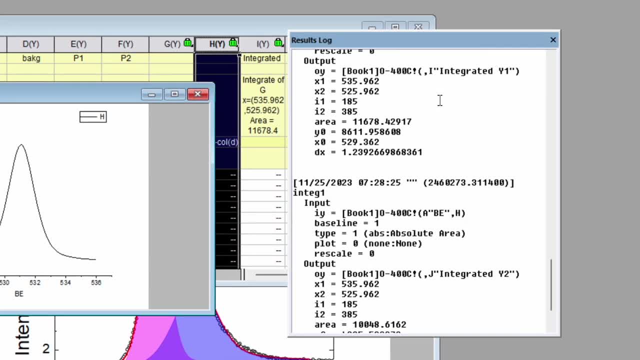 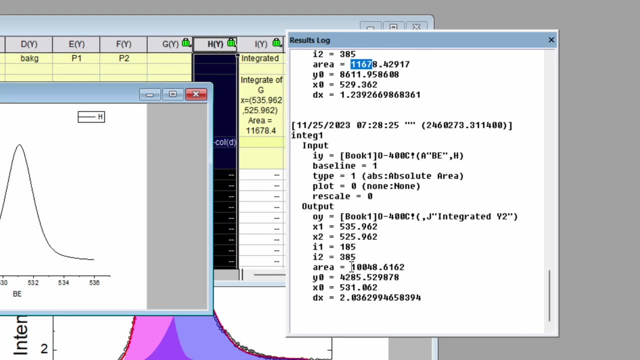 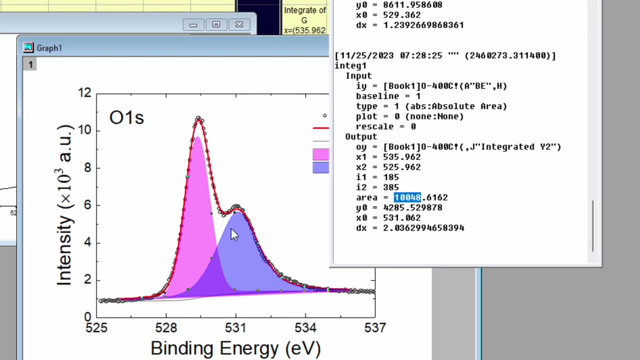 We can see the results. So the first peak area is 11678, whereas the second peak area is 10048.. That's all. So from this we can confirm the area of the pink curve has a higher contribution to the XPS vector than the blue one. 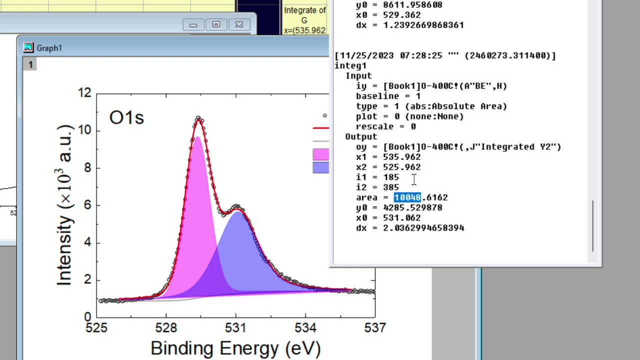 And the total number we can get from these numbers. I hope through this video you learn how to calculate area under curve in origin software. Do like, share and subscribe. Press the bell icon button to be updated with my new videos.